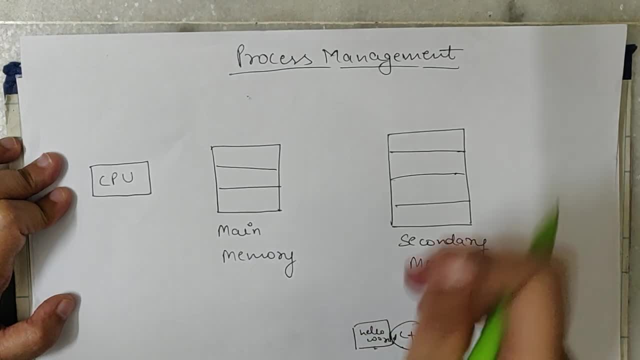 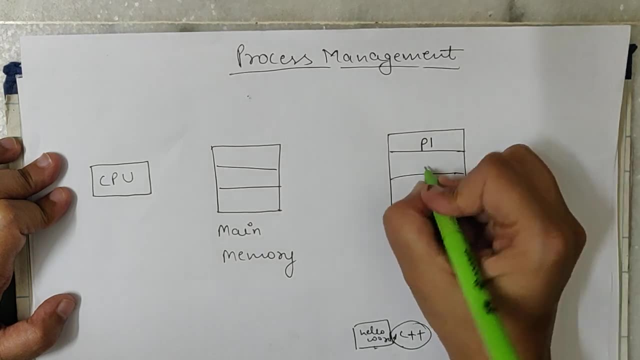 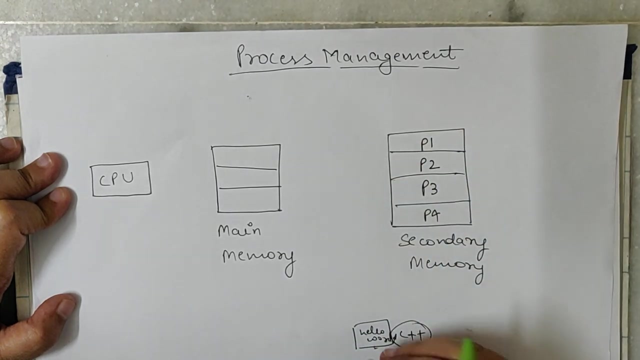 p1. I have saved this hello world program inside this secondary memory and let's say the program's name is p1. i have made another program, let's say p2. I have made another program, p3, p4 and so on, and all these programs I have made. 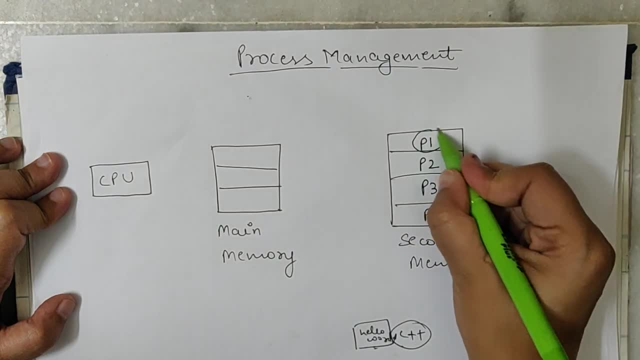 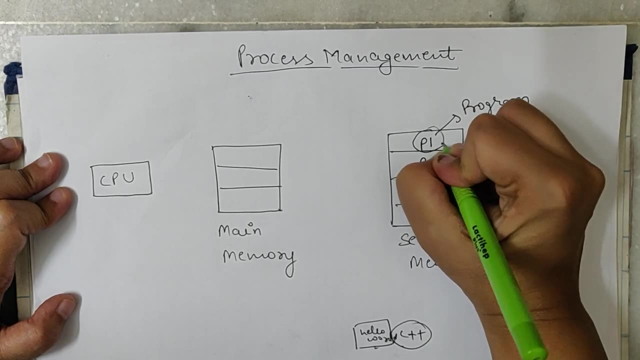 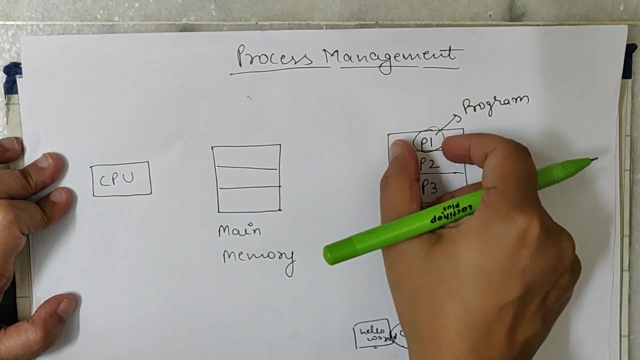 will be saved in the secondary memory. so what is this known as program? okay, if I want to execute this particular program, I reside in the main memory. CPU will execute my program P1.. So for the execution, this program P1 should be reside in the main memory. So what operating system does is move this. 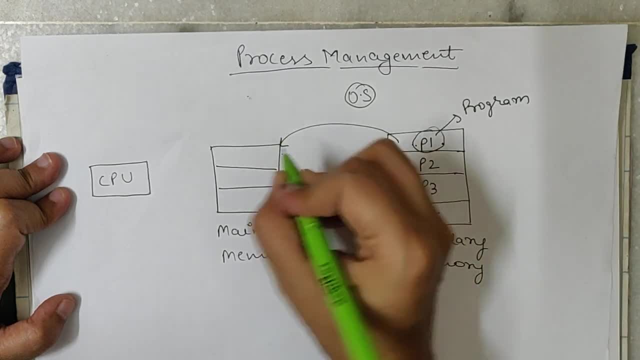 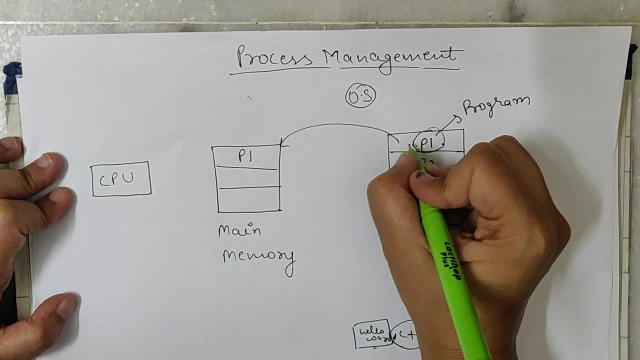 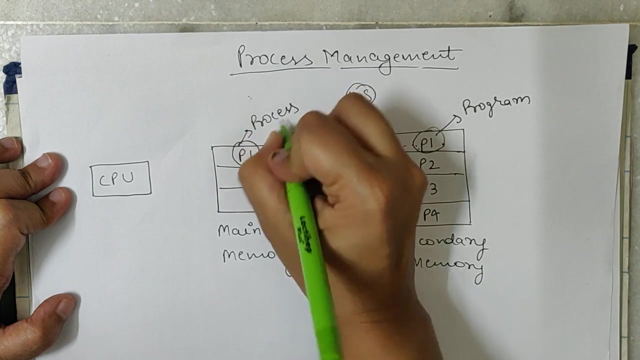 program P1 inside the main memory like this: Once this program moved inside the main memory, this is known as process. The same program which is moved from the secondary memory to main memory is now known as process. It is not known as program, it is now known as process. 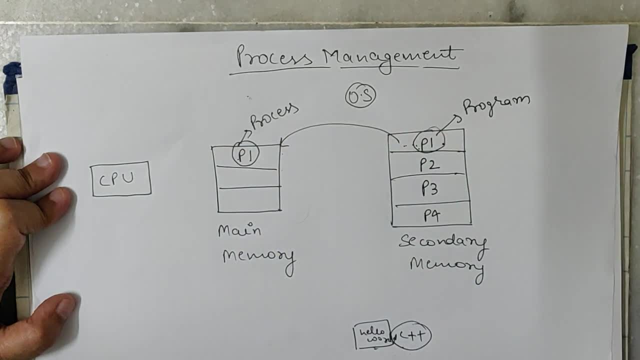 Ok, now CPU picks this process and executed it. Ok, so when the program is inside the secondary memory, it is known as program. Once it is moved to the process, it is known as. once it is moved to the second, from secondary memory to main memory, this program is now. 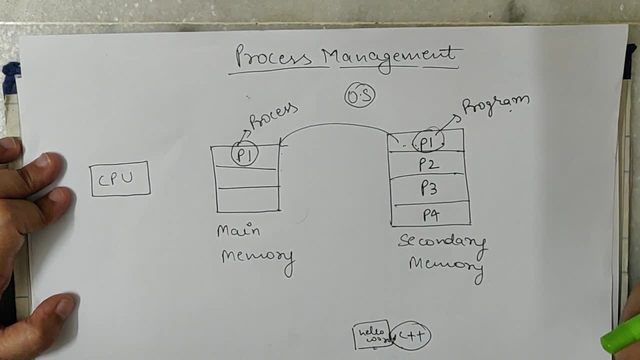 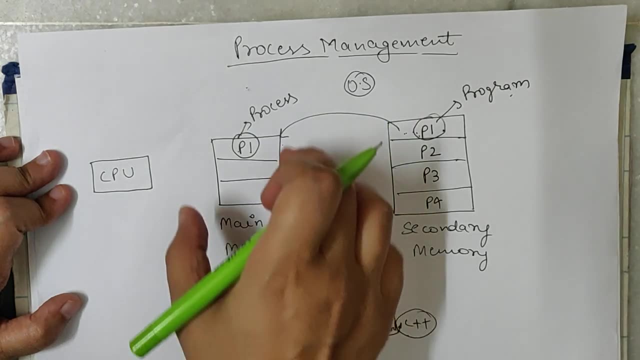 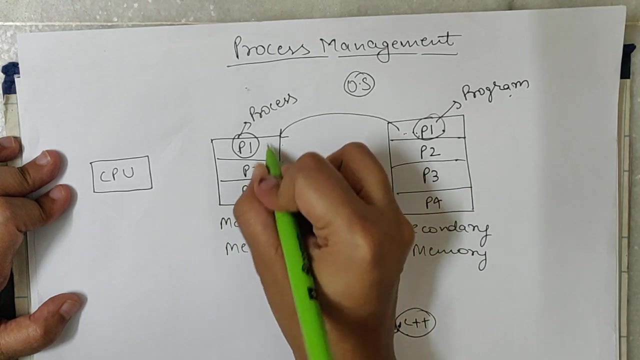 known as process. So program under execution is nothing but process. So actually operating system manages all these processes inside the main memory. Ok, say suppose I have moved this program P2, then P3. So all these programs want, we want. 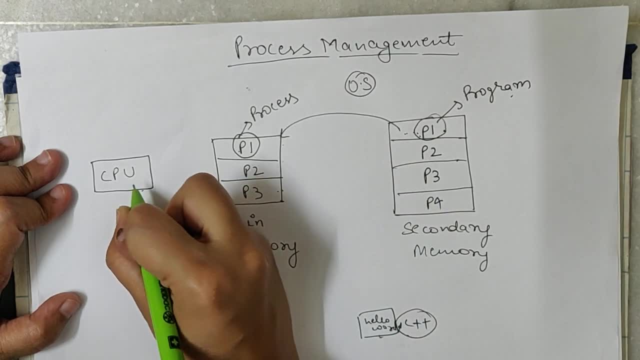 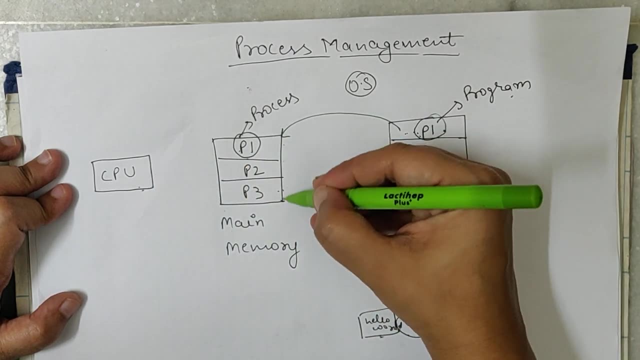 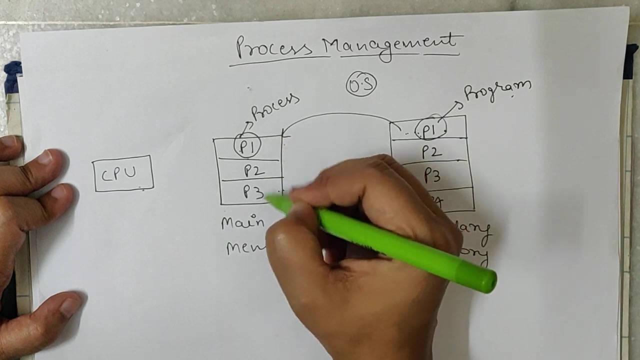 these programs to execute by the CPU. CPU will execute one process at a time because CPU is only one, so one process at a time it will execute. So all these processes are in the waiting state, are ready for execution. They are waiting for the CPU. They all want to access the CPU and CPU is only one and they 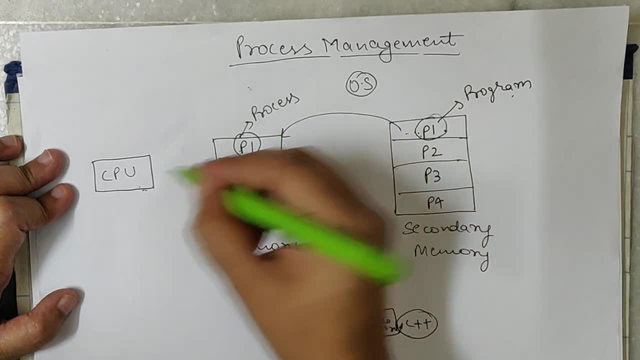 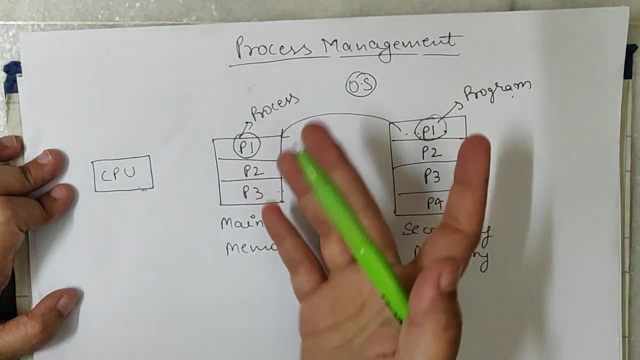 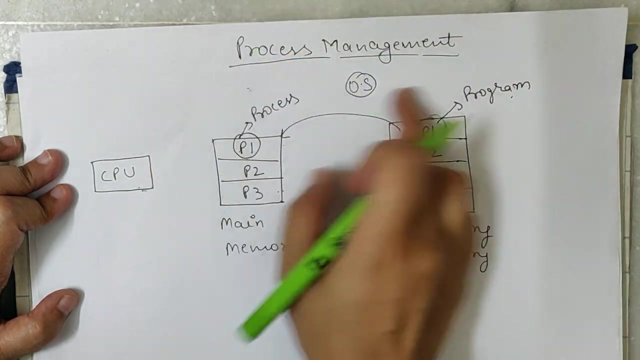 all want to access the CPU. So one by one they will get the CPU. So operating system manages all the processes. Who will get the CPU first? Who will get the input output resources? All these is managed by the operating system. So this all comes. 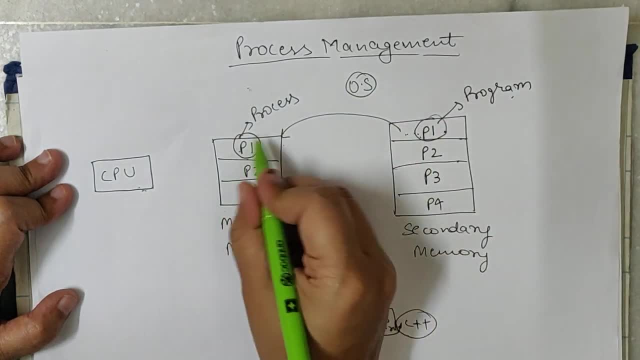 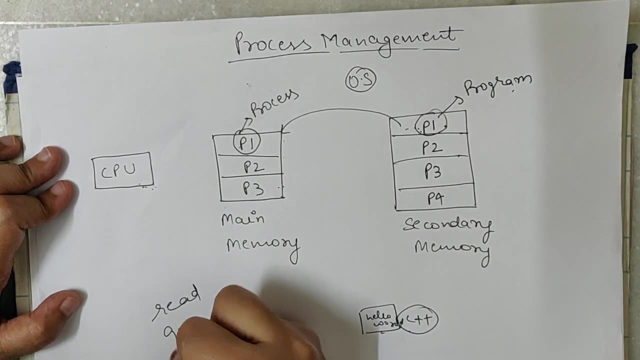 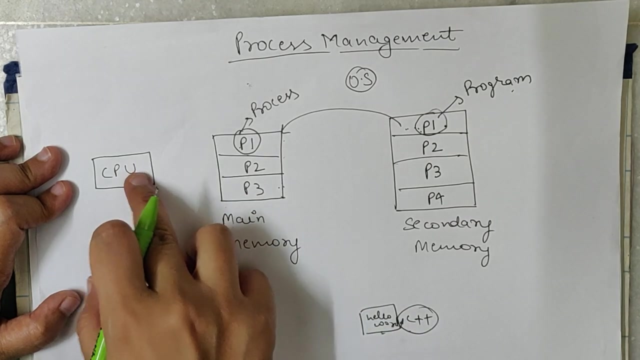 under process management. Ok, So all the processes inside the main memory are waiting for the CPU. So we have a ready queue data structure. In this ready queue, all the processes are waiting for the CPU. This is a data structure. QQ means they are all. 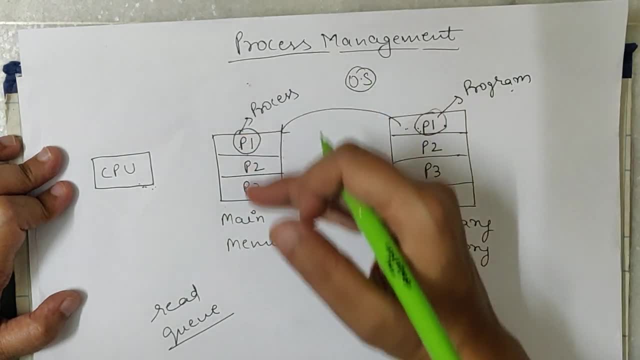 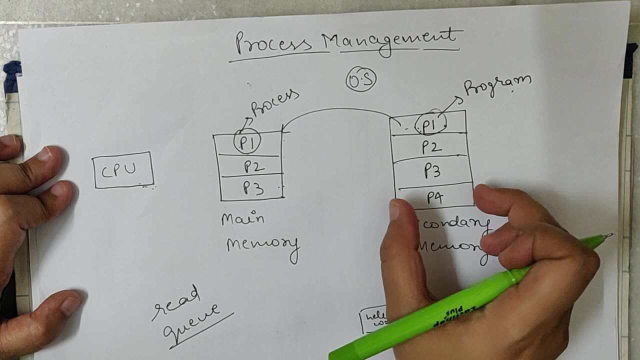 waiting in a line 1 by 1, P1, P2, P3. they are all waiting in the line for the CPU. These are the programs. If we want to execute these programs, they has to reside in the main memory. Once they are reside in the main memory, 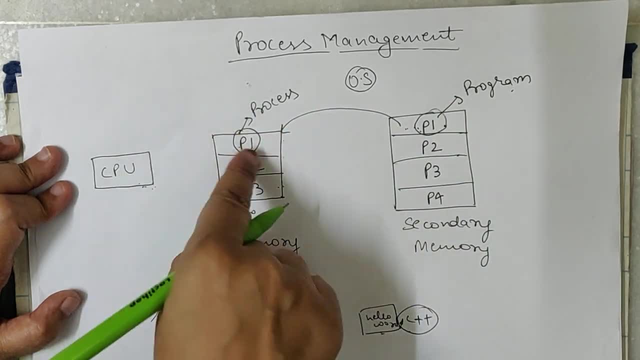 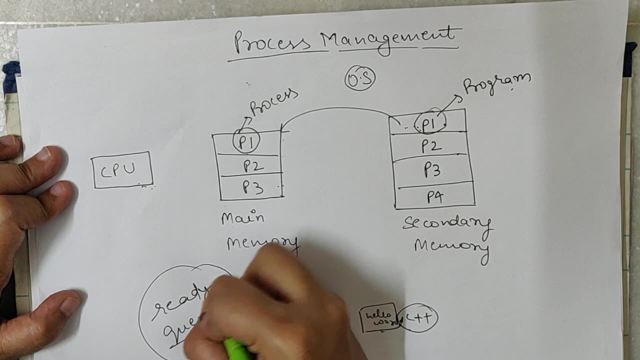 they are known as process, and CPU picks up 1 by 1 each process for the execution and these process are in the waiting state. They are ready for execution and they are waiting inside the ready queue. They are all waiting in a line. Therefore it is. 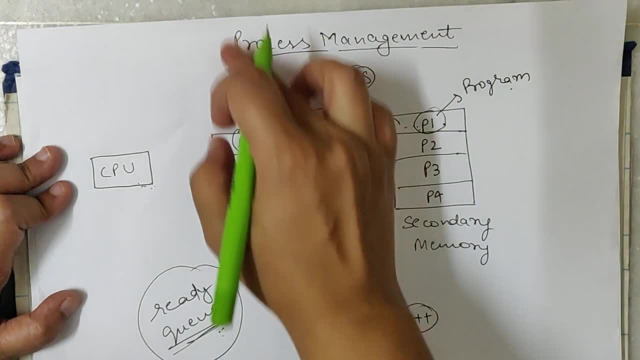 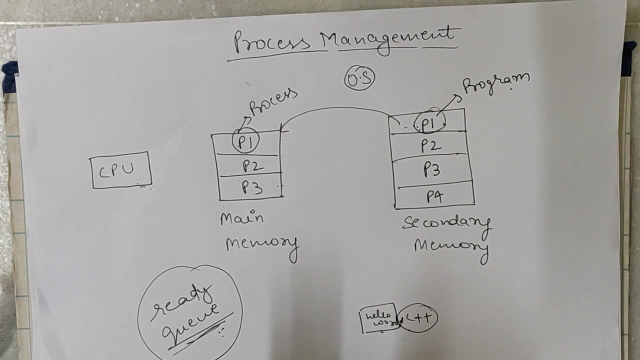 known as queue. Queue is nothing but a data structure, So all this is managed by the operating system. This is just a gist of process management. We will discuss it in detail, but I hope this is clear now: what is a program, what is a process and how? CPU? 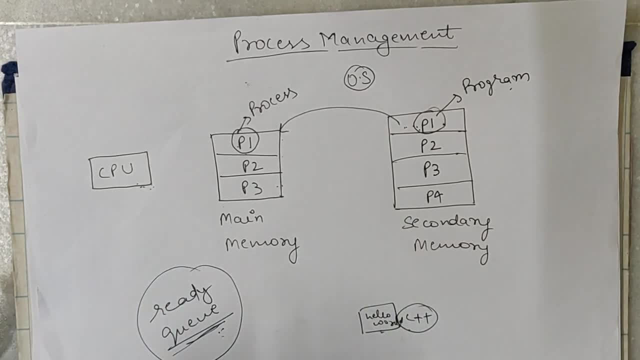 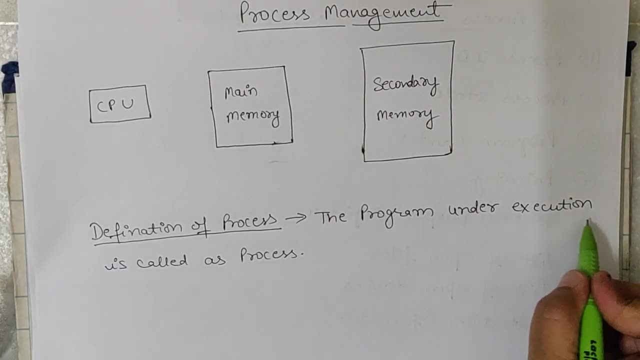 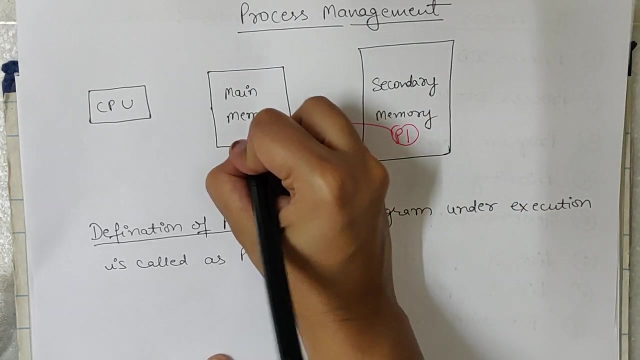 picks the process from main memory for the execution. Ok, So the formal definition of a process is the process. the program under execution is called as process. Ok, This is a program P1 when it moves inside the main memory. Now, this is a program. 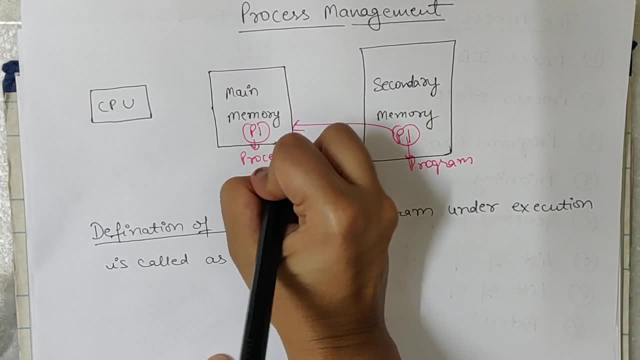 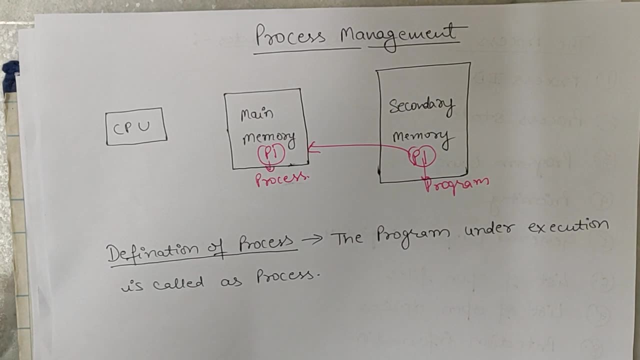 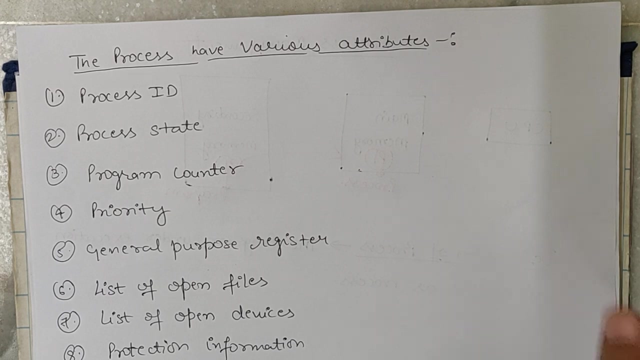 from the secondary memory to main memory. it is now a process and now CPU picks this process and execute it. Ok, So process has various attributes. Like human, we have our Aadhar ID, our address. Like process also, they have attributes like process ID. Each process has its own. 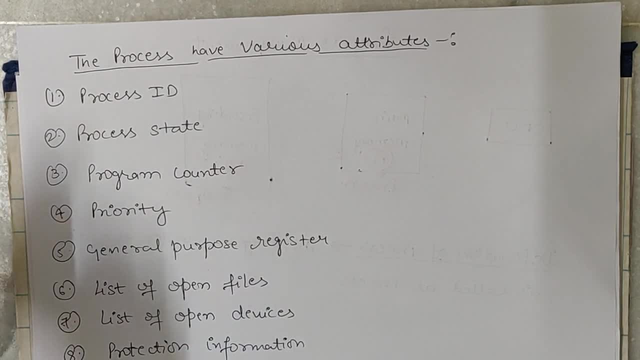 unique ID. Process state means it is under with state, New state, ready state. I will explain this process state in next tutorial. So process state means currently it is in ready queue or it is executing the CPU. What actually it is inside? 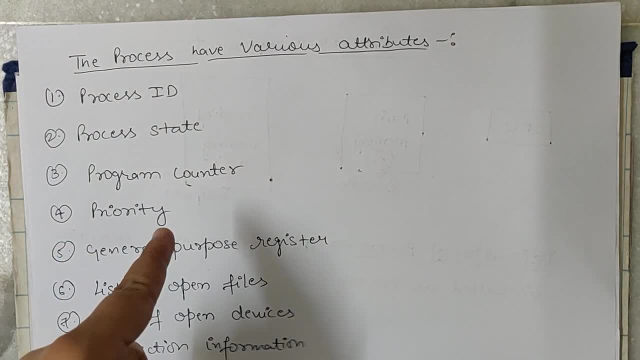 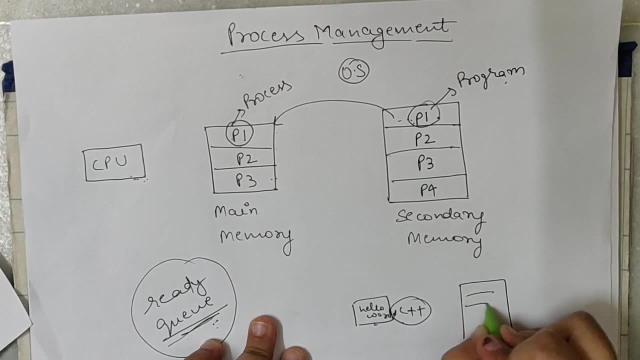 it is in the current state. Ok, Program counter means you have a process. Ok, Now there is a program, so it will have a lot of instructions. Ok, This is my program P1 and it has lot of instructions and each instructor. 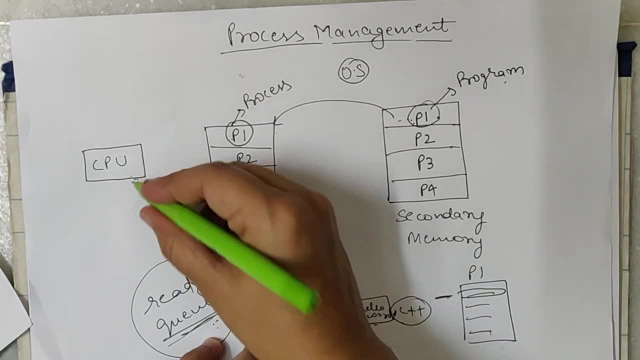 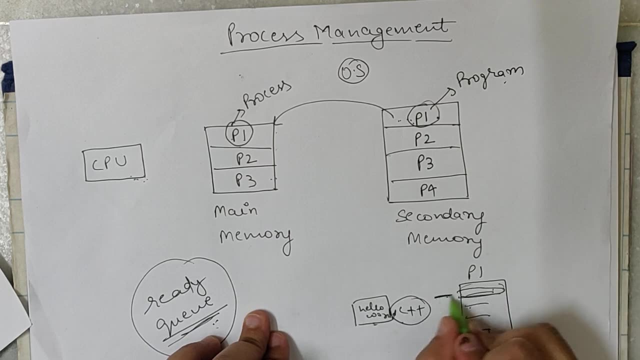 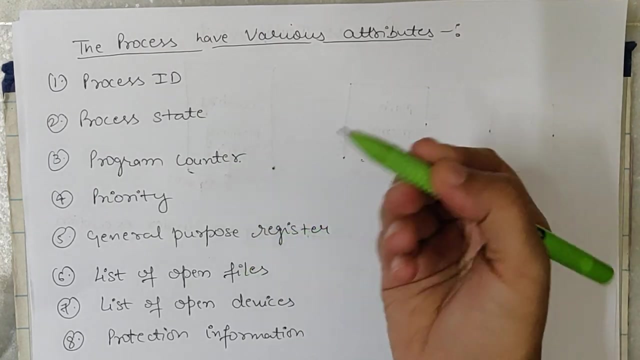 instruction has a address. Ok, So CPU picks one instruction, executed it. Then picks up the next instruction, then executed it. So each instruction has its own address. So the program counter stores the address of the next instruction. CPU will find out the address of the next instruction from the 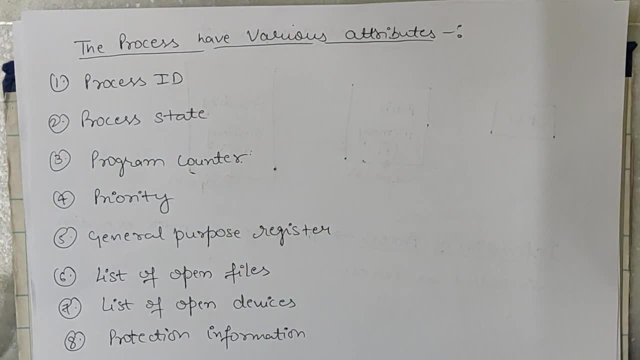 program counter. Ok, Next is the priority. Priority means operating system sometimes assigns the priority to each process, Like it is a high priority process, So CPU first picks up that particular process which has higher priority. Ok, So this also I will discuss in CPU scheduling algorithm General. 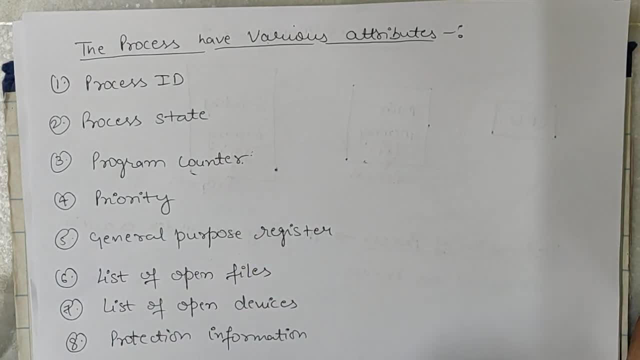 purpose. registers means what kind of registers a particular process holds. List of open files means what are the files it is used. the particular process is using The number of files the particular process is using. List of open devices means what kind of devices the particular process is using, For example, a. 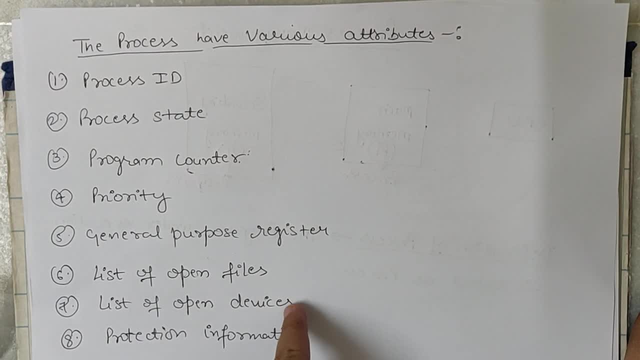 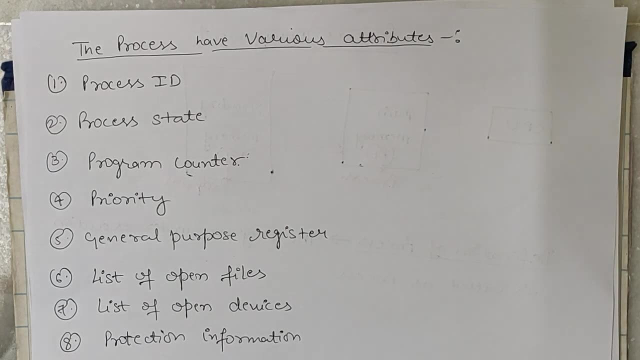 particular process is currently using a printer. So it is it is a printer, it is using printer. Then the protection information in this it is, if any case, mechanism. So protection information is if a process is using some protection, it is that information is present. 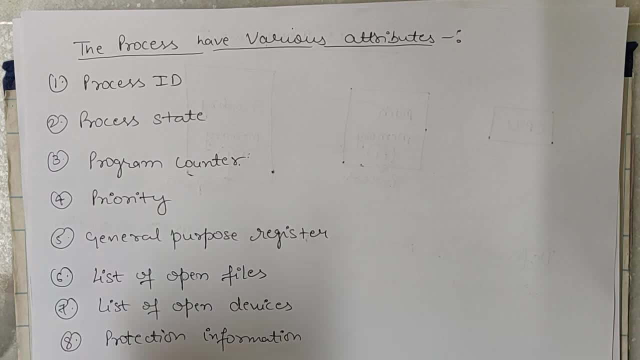 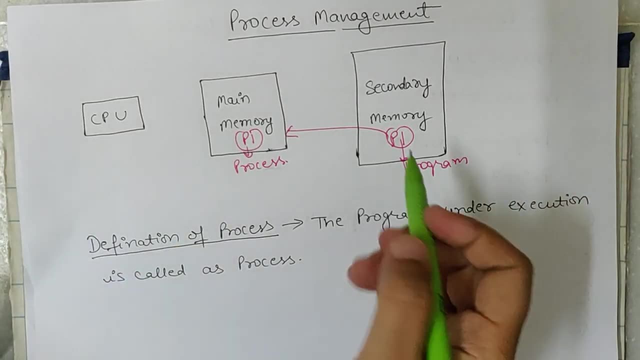 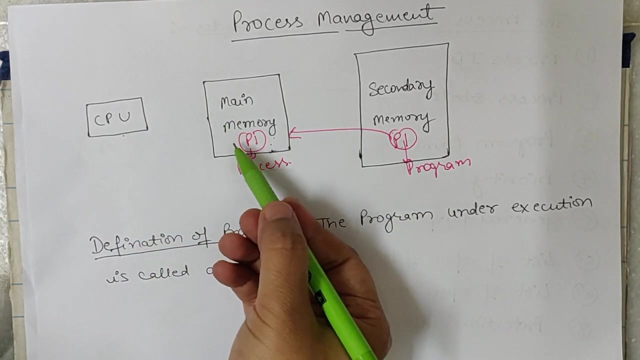 inside, maintained inside this protection information attribute. So these are. these are some various attributes of a particular process. now, who will picks up this program to from the secondary memory to main memory, and who will picks up this process? who will assign the CPU to a particular process? this is all done by scheduler, CPU schedulers. so 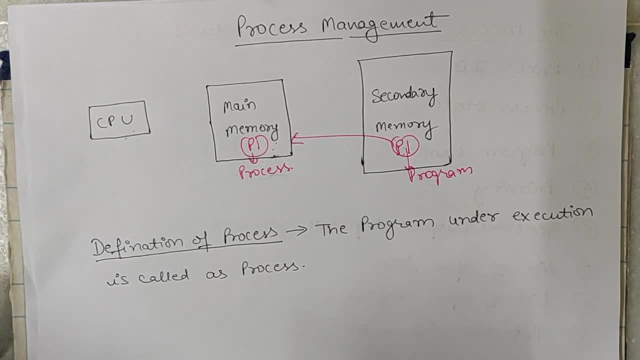 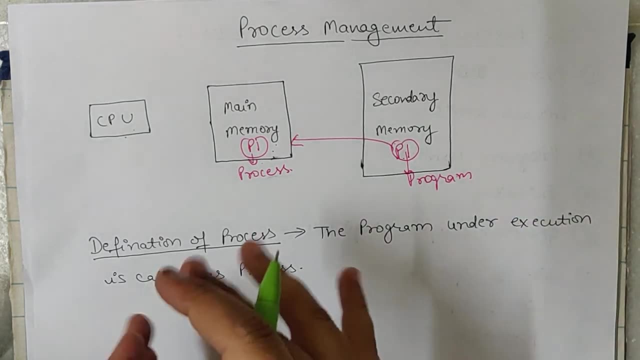 what are the? what are schedulers and what are the types of schedulers we will discuss in the next tutorial. I hope the term process and the types of attributes of the process is clear now. I will discuss the types of schedulers in the next tutorial. thank you so much, please.